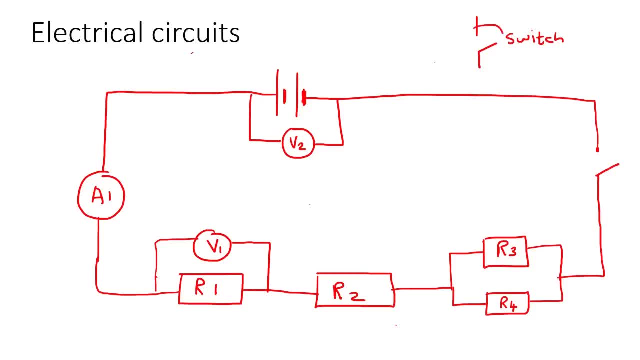 when you switch your lights on, that's a switch. So when the switch is like this, we say that the switch is open And what that means is no electricity is able to flow. So this is where you would switch your lights off, for example. that's what it would look like. 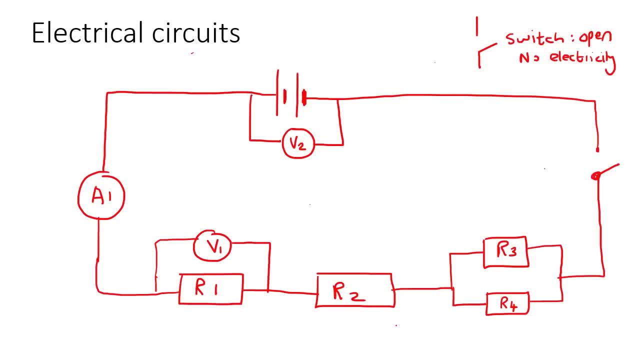 Now, if you decide to close that switch, so let's close the switch now- then all you do is it'll look like that, And so when you have it, you're going to have a switch. Now, if you decide to like that, well then the switch is closed And now it means that there is electricity. So 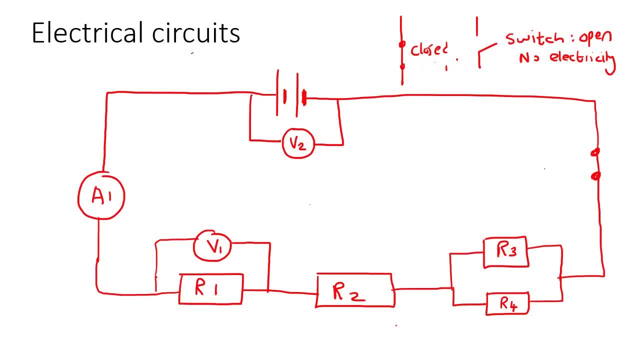 electricity. well, let's say here, electricity is flowing Okay, And so that's the first thing I want to talk about. So now that the switch is closed, electricity is going to start flowing. So the next thing I want to talk about is this part over here. you see this part. 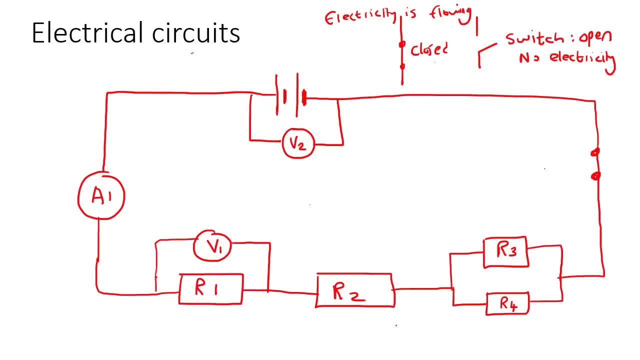 whoops, that has a long line and a small line. Now, that part there that has a long line and a small line, well, the long line is the positive and the small line is the negative, And that is called a cell. Okay, Now, if you put more than one cell next to each other, so there, 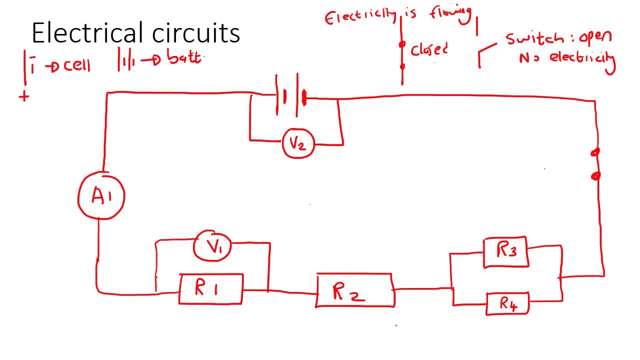 we have two cells, then we call it a battery. Now the battery is so important. The battery is what gives the electricity, The energy that it needs to be able to flow. So it gives the electricity, or let's rather say it gives. it gives energy to the charges. Now, remember, electricity is charges that are busy moving. Okay. 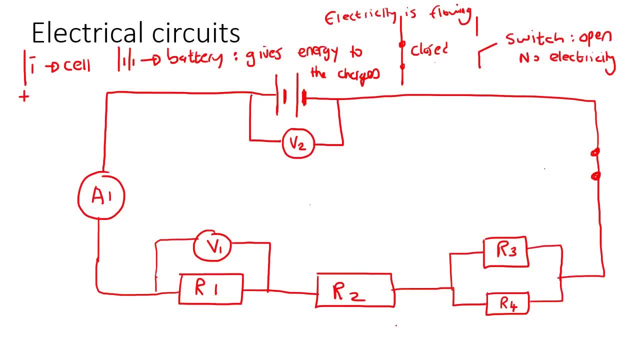 It's actually electrons, but let's just call them charges for now. So the battery is what gives the energy. It's actually electrons, but that's a charge. that's not necessary, But let's just call them charges. So the battery is the current. the current is the current energy that is flowing in the battery. 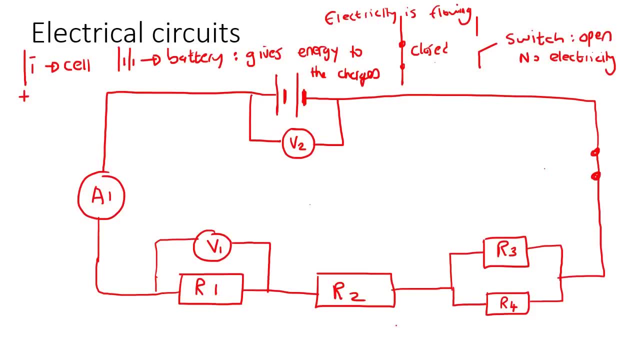 And the current energy has to get blocked to the battery. So the battery has to get blocked to the battery. It has to go through the electricity and the current is going to get blocked. So of course, electricity is going to get blocked very, very, very quickly. 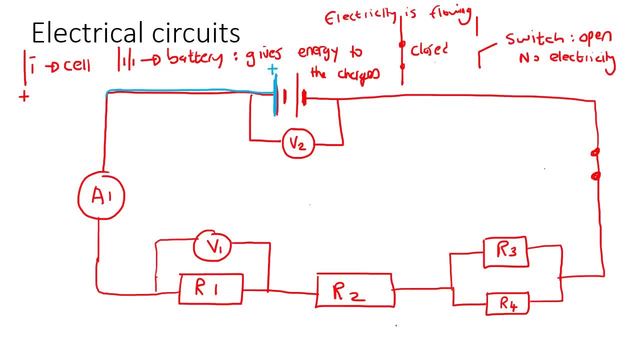 So there's all the other components involved here in this, So the power will be there. Okay, it's right there in the circuit. It's not a power unit or a voltage. It's not a power unit, It's a current. 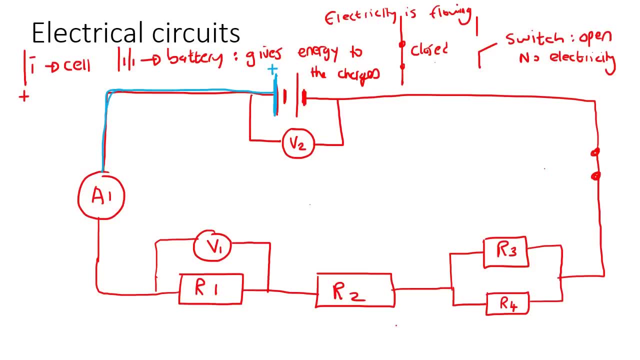 It's a current Okay, reach this device which is called an ammeter. this device, which has a little a, is called an ammeter, and what an ammeter does is it measures how much electricity is flowing. how much electricity is flowing, that is what the ammeter does. 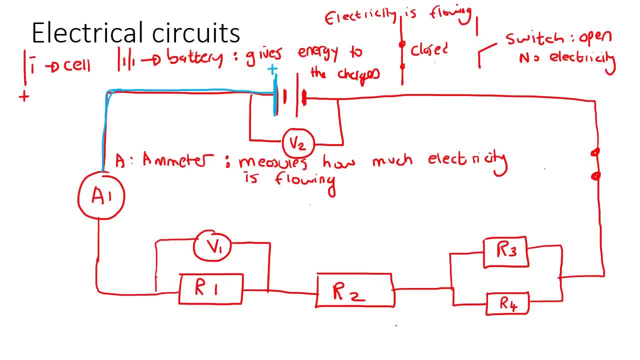 but it does not, um, or it's very easy for the electricity to go right through the ammeter. you can almost think of the ammeter like a bridge and the cars are just going under the bridge, so the bridge doesn't get in the way of the cars. okay and um, what happens is that the electricity keeps. 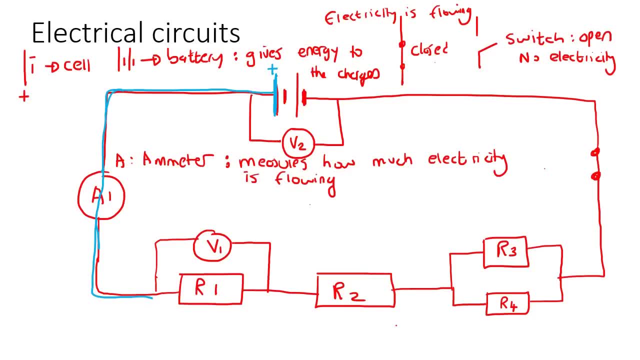 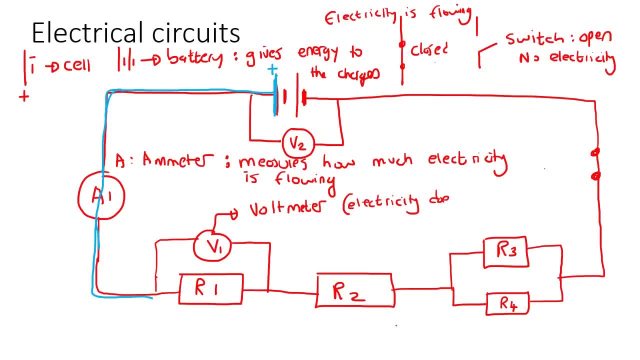 a voltmeter. electricity does not flow through a voltmeter, okay, and so what a voltmeter does? let's also talk about that. it measures: how much energy is the charge or are the charges using? how much energy are the charges using? okay, i'll explain a bit more about that now. so what happens? 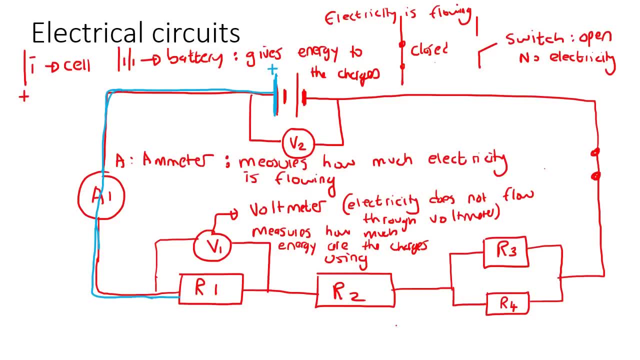 that the electricity goes this way over here and suddenly it starts going through a device called a voltmeter. okay, and so what happens is that the electricity goes this way over here. r now the one in the, the r1, r2, r3, that's just to say the different r's, like each, each one is. 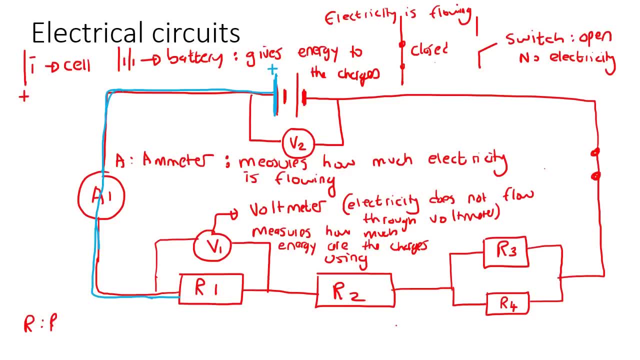 different, but an r is called a resistor. now, a resistor can be anything. it could be a light bulb, it could be a television, it could be a fridge, it could be any type of device that you need to switch on, for example. okay, okay, and so all i want you to know so far is that the battery is what gave the energy. so the battery. 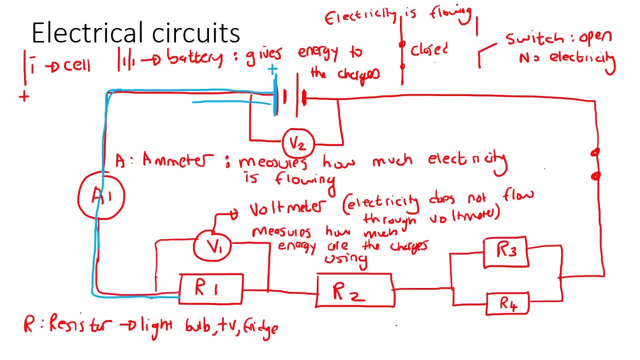 gives the energy to the charges. the charges then start moving through the circuit and they use the energy to be able to go through the different resistors. now the v is just something that will tell us what will measure how much energy was used. okay, that's all that you need to know so far. 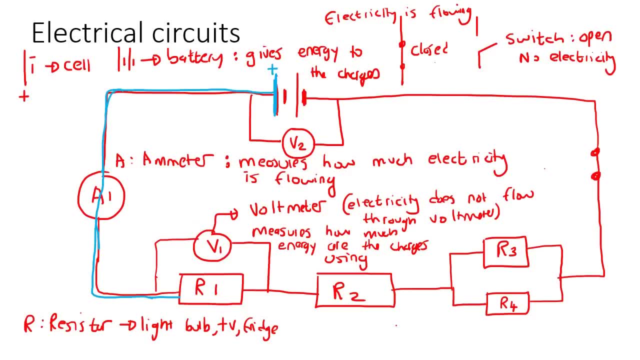 so this voltmeter is connected to a voltmeter. so this voltmeter is connected to a voltmeter over here and over here. so it will measure how much energy is used when the electricity goes from here up to here. so it just measures how much electricity, how much energy is used over there. 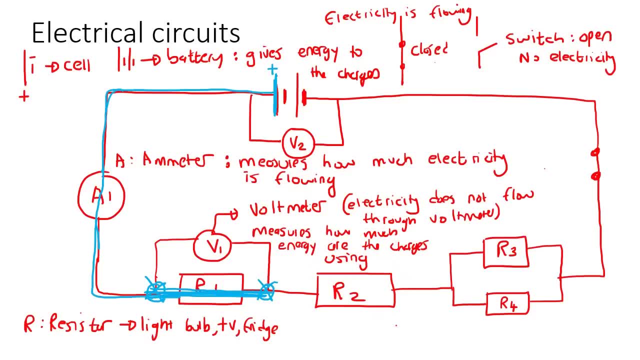 okay, it does not measure how much energy was used there. and it does not measure how much energy was used there, it only measures how much energy is used in that device over there. so then, kevin, why don't we also connect one over here? well, we could if we wanted to, but maybe the people who built the 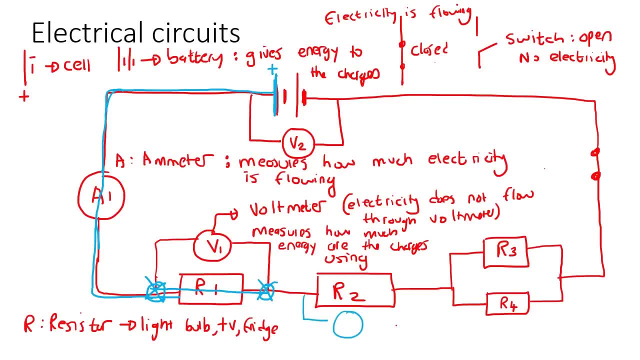 circuit decided that they just don't need to know how much energy was used over here. maybe they don't want to know, but if they wanted to, they could just go build another voltmeter and they could call that one v3 if they wanted to whoop, they would rather connect it there, and then they would be able to. 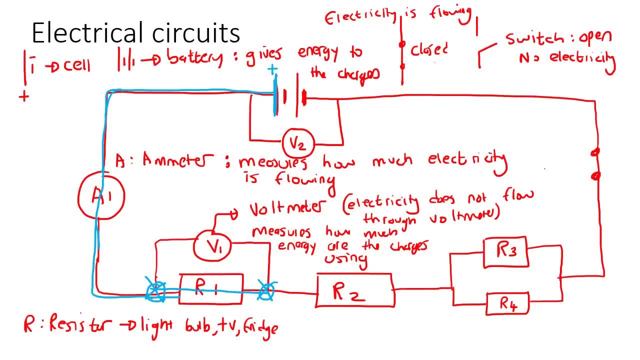 measure how much is used. okay, so the electricity keeps flowing. and now it goes through r2. maybe r2 is a different type of device and it's a different type of device and it's a different type of device. maybe it's a microwave, or a kettle, or a toaster, or another light bulb. we don't know, it could be. 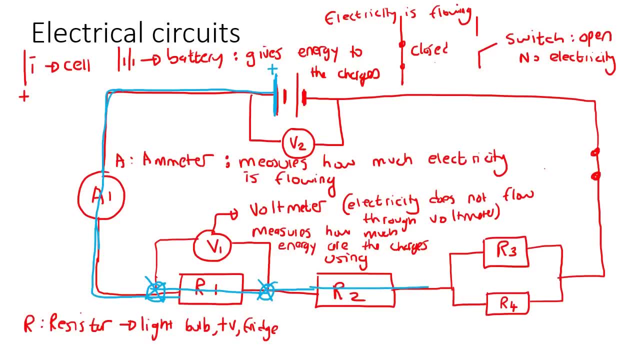 anything, but the electricity flows through it like that. okay, now i want to stop there and just talk about something. can you see that the electricity went through this one and it went through this one straight after each other, so we will say that r1 and r2 are in series. 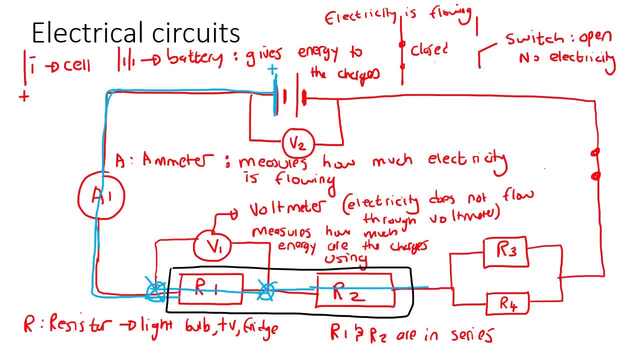 series means that they go, that the electricity goes through both of them straight after each other. okay, so they are in series and we'll talk about that in detail in future lessons. right? so what happens now is that this electricity gets over here now. now, here it needs to make a decision. what happens is that some of it is going to go. 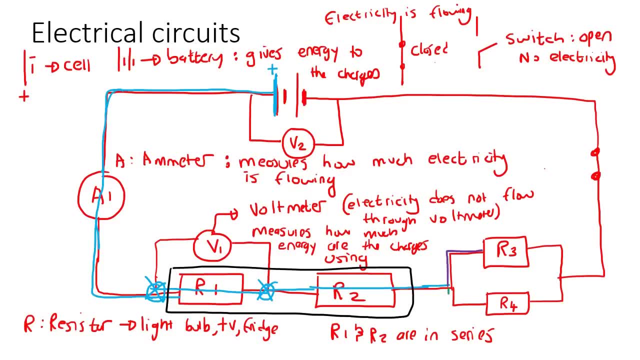 this way, and some of it is going to go this way, so that'll go through r4- maybe r4 is another light bulb or something like that- and then it'll get here and then some of the rest will go through r3 and then it'll all come together over here again and then it'll join to become the same. 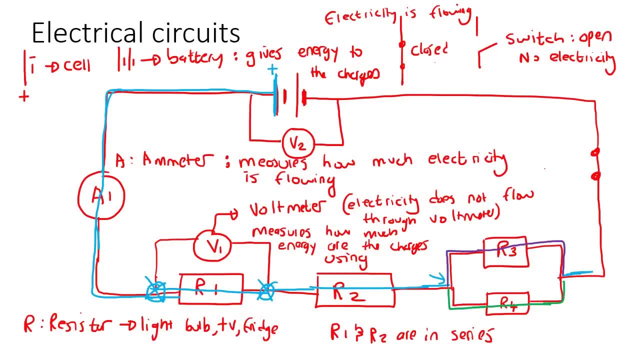 amount of electricity that we had before we got to this part. so let's just talk about that again. so here we've got a whole lot of electricity that's busy flowing. okay, maybe we have 100 charges, maybe we have a hundred. you can think of a hundred small little electrons that are busy. 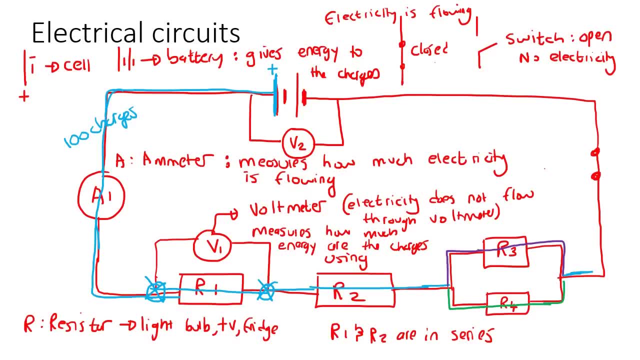 flowing and they bought. they're all flowing nicely together and then what happens is 100 of them go through here and 100 charges went through here, but then all of a sudden, they get to this part. now some of them are going to go this way and some of them are going to go this way. 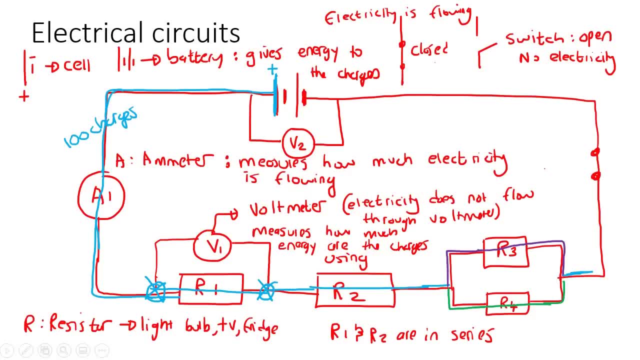 and some of them are going to be 50, 50. well, sometimes, but not always, and we'll get to that in later lessons. so let's say 40, go this way, and let's say 60, go this way. then what happens is when they join up, 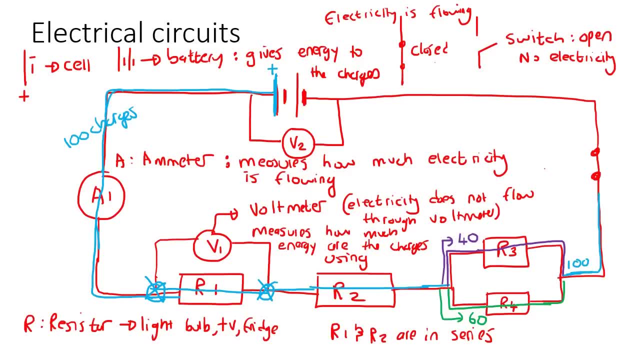 together again, they will have 100, and then those 100 charges will carry on all the way around. so one of the last things i want to talk about is that when you look at this ammeter, what does this ammeter do? it measures how much electricity is flowing. so how much electricity was flowing over here? well there, 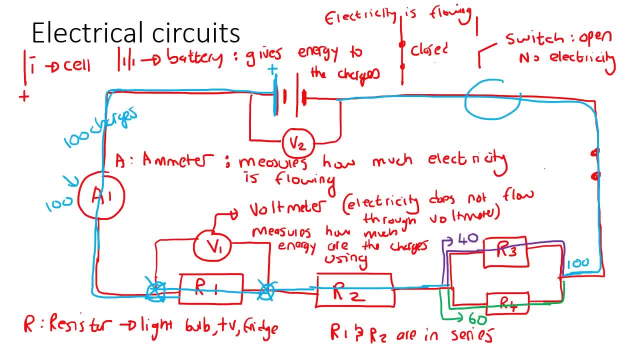 was a hundred, how much electricity would be flowing over here? well, that would also be 100, wouldn't it? and so if we had to put another little ammeter over here, that one would also measure 100. what if we had to put an ammeter over here and we would call that one a3? well, that would also measure. 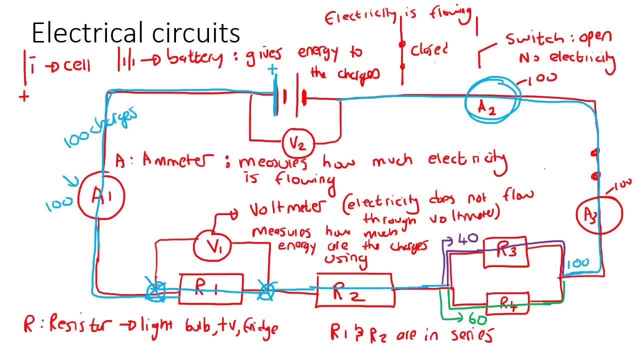 100. but if we had to go put an ammeter over here and we could call that a4,, well, that would only measure 40,. and if we had to go put an ammeter over here, maybe we could call that one a5,, well, that one would only measure 60,. okay, and so.